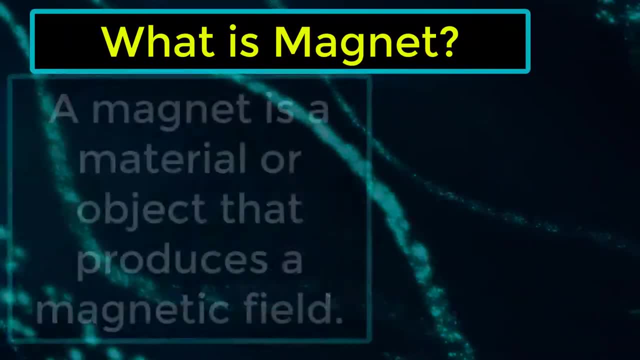 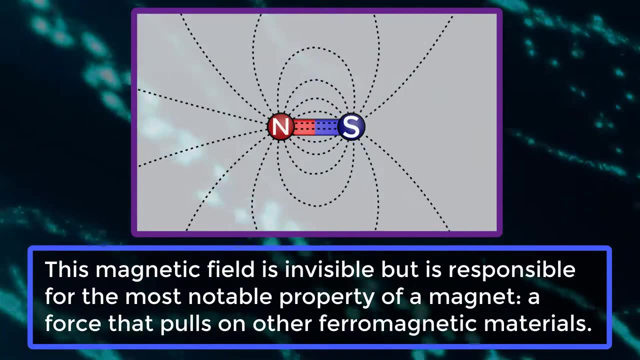 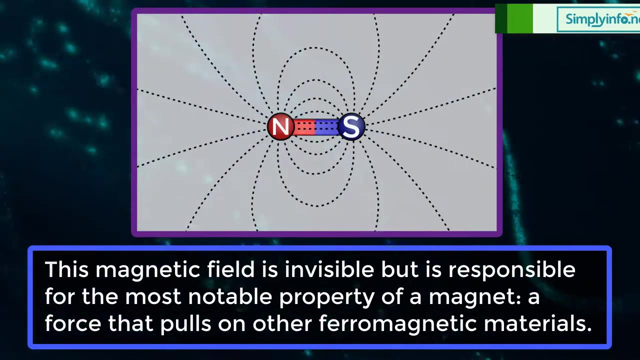 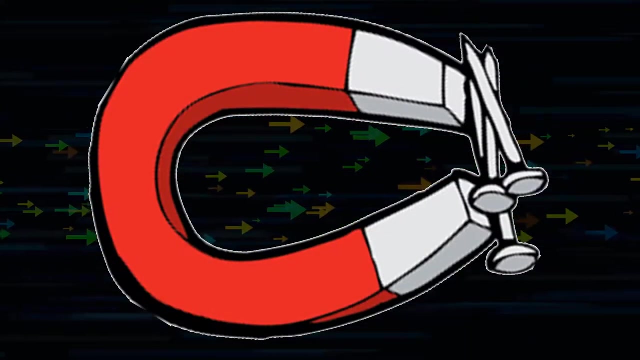 What is magnet? A magnet is a material or object that produces a magnetic field. This magnetic field is invisible, but is responsible for the most notable property of a magnet. That is, a force that pulls on other ferromagnetic materials, such as iron, and attracts or repels other magnets. A permanent magnet is an object made from a material. 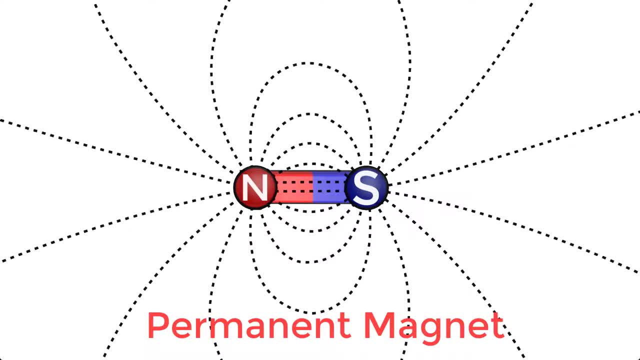 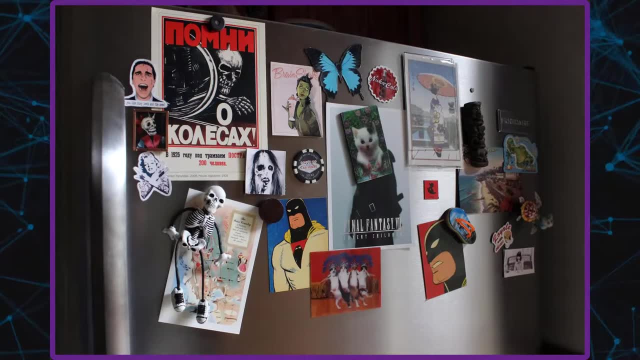 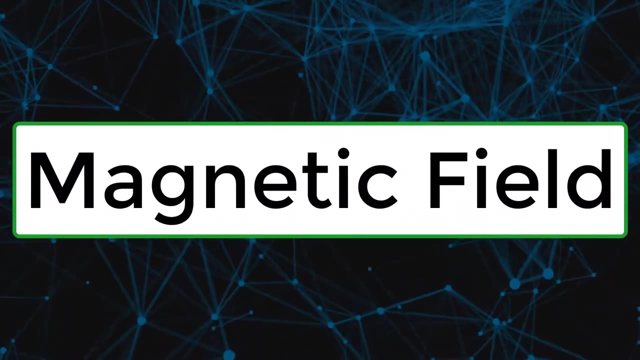 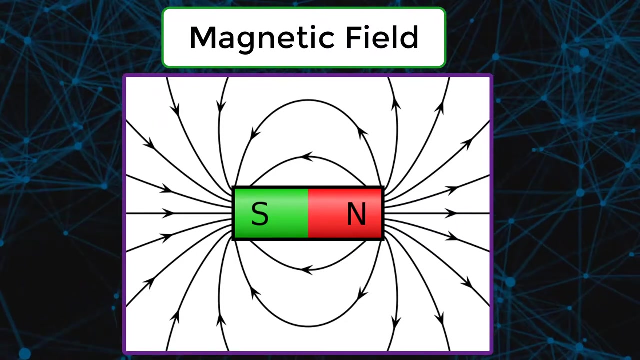 that is magnetized and creates its own persistent magnetic field. An everyday example is a refrigerator magnet used to hold notes on a refrigerator door. Now let's look into magnetic field. A magnetic field is a vector field that describes the magnetic influence of electrical currents and magnetized materials. 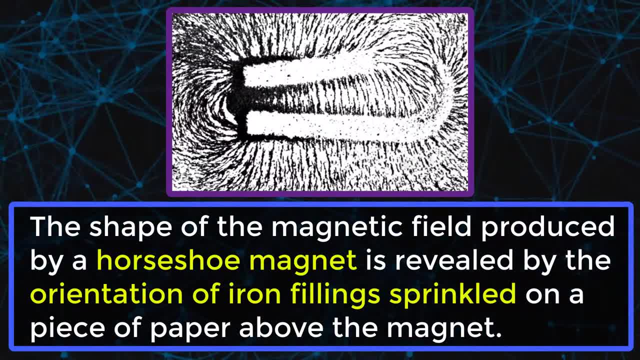 The shape of the magnetic field is a vector field. The shape of the magnetic field is a vector field. The shape of the magnetic field produced by a horseshoe magnet is revealed by the orientation of iron fillings sprinkled on a piece of paper above the magnet. 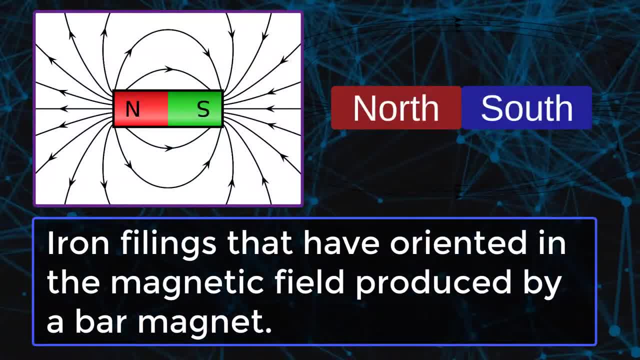 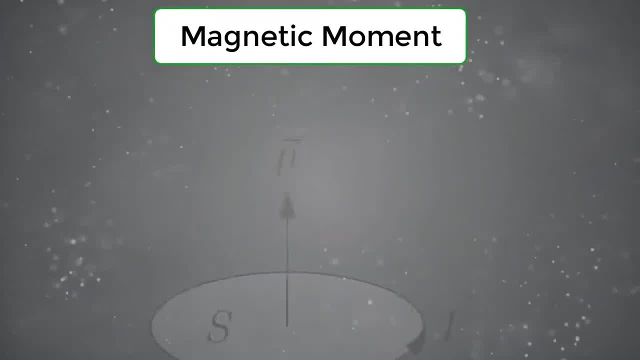 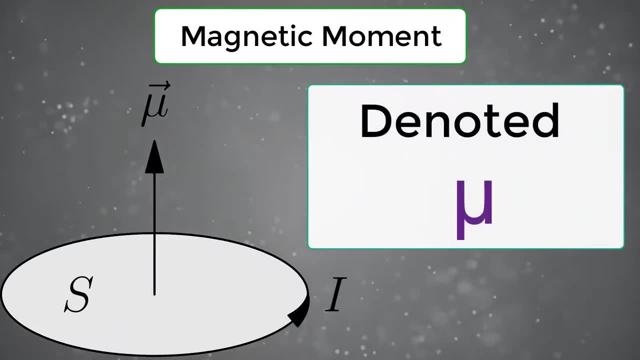 Iron fillings that have oriented in the magnetic field, produced by a bar magnet. Now, what is a magnetic moment? A magnet's magnetic moment, also called magnetic dipole moment and usually denoted mu, is a vector that characterizes the magnet's overall magnetic properties. 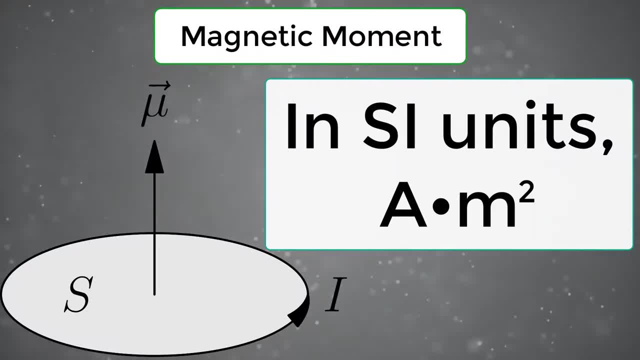 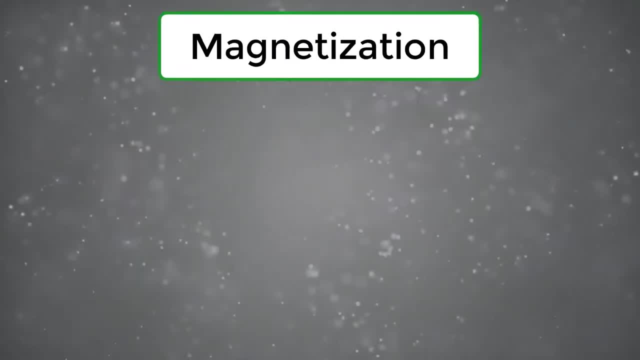 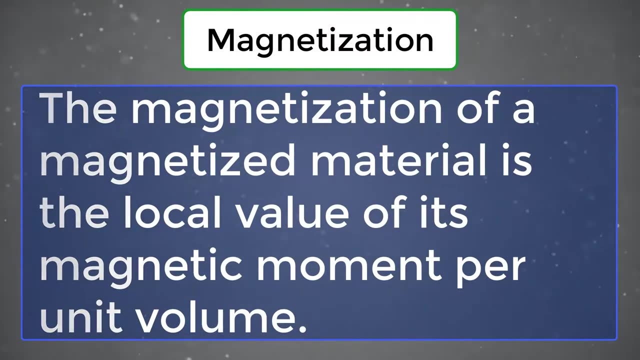 In SI units the magnetic moment is specified in terms of amperes times meter. squared Magnetization. A magnetization of a magnetized material is a local value of its magnetic moment per unit volume, usually denoted m, with units ampere meter. 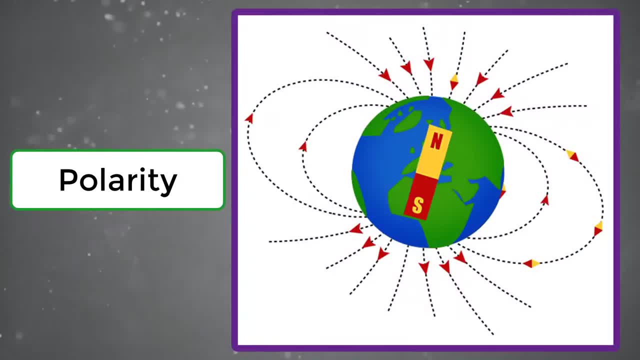 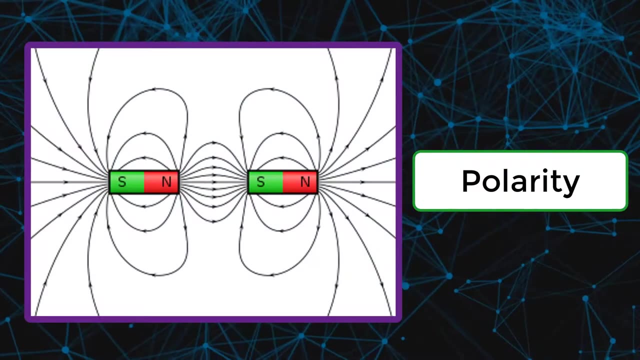 Polarity. The north pole of a magnet is defined as a pole that, when the magnet is freely suspended, points towards the earth's north magnetic pole. in the Arctic The magnetic and geographic poles do not coincide, see magnetic declination- Since opposite poles- north and south- attract.